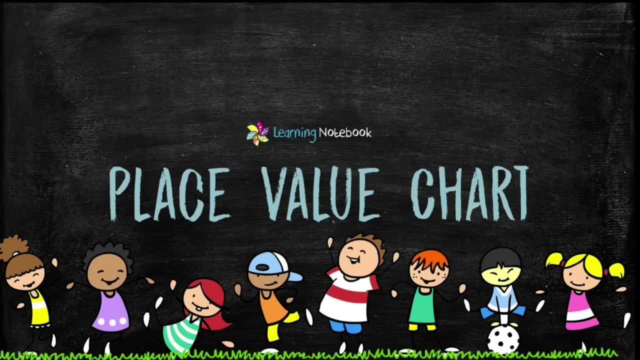 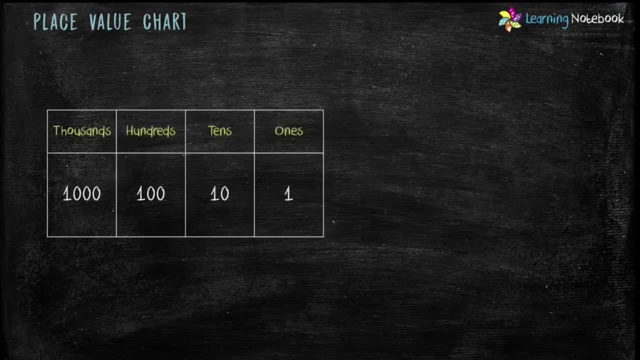 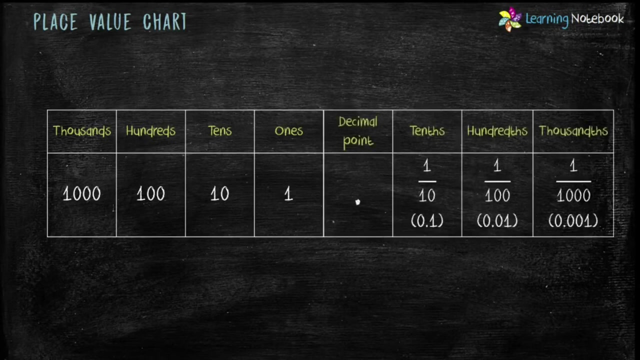 Now let's understand the place value chart of decimal numbers. Students, we already know the place value chart of whole number, which is 1,, 10,, 100, 1000 and so on. Now the place value chart of decimal part of decimal number is 10, which is 1 by 10 or 0.1.. Next is 100. 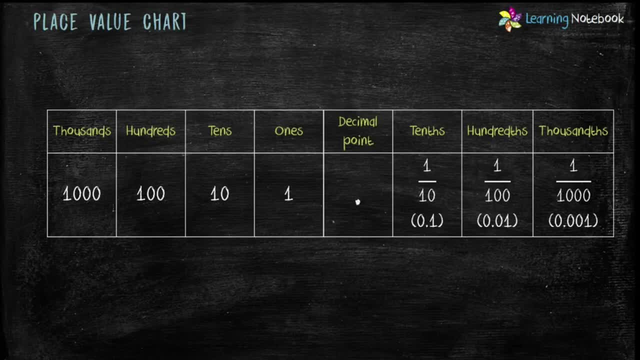 which is 1 by 100 or 0.01.. After that 1000, which is 1 by 1000 or 0.001, and so on. So the whole number part has two parts and the decimal part is 100.. 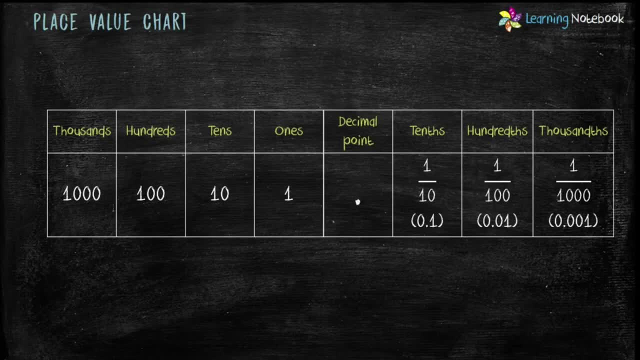 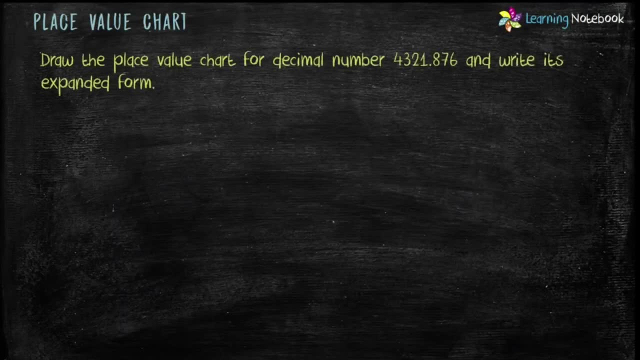 This entire table is the place value chart of decimal numbers. Now let's draw the Place Value chart for decimal number and write its expanded form. Decimal number is 4321.876.. First let's make a place value chart of whole number part. 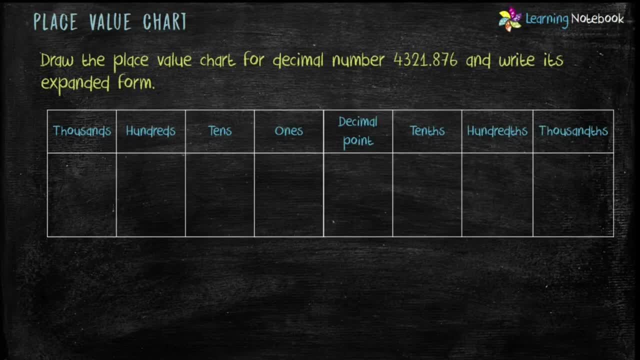 which is 4321.. Decimal number is 4,026.. This entire table is the place value chart of decimal numbers. So let's put 1 at 1's place, 2 at 10's place, 3 at 100's place and 4 at 1000's place. 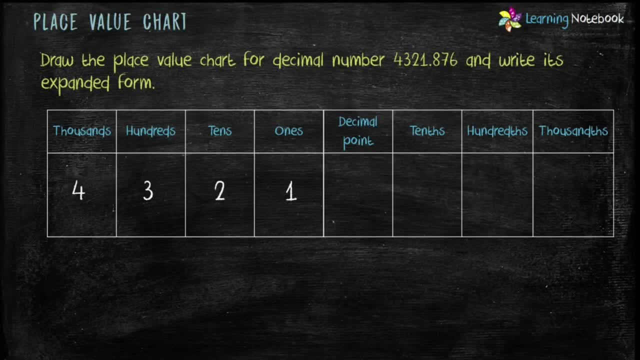 Let's start with the decimal part. now Put a decimal point, then write 8 at 10's place, 7 at 100's place and 6 at 1000's place. This is the place value chart for the given decimal number. 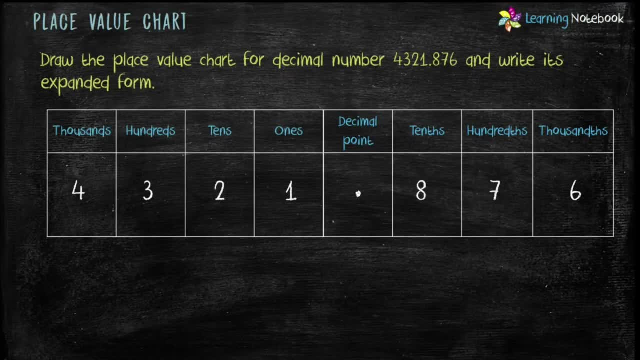 Now let's write its expanded form. To write expanded form, we first need to find the place value of all the digits. Place value of 1 is 1,. place value of 2 is 20,, 3 is 300 and 4 is 4000. 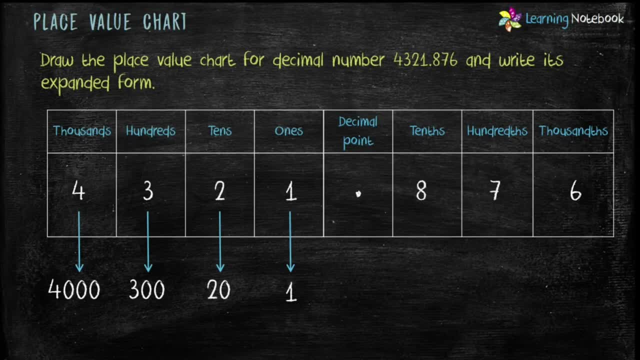 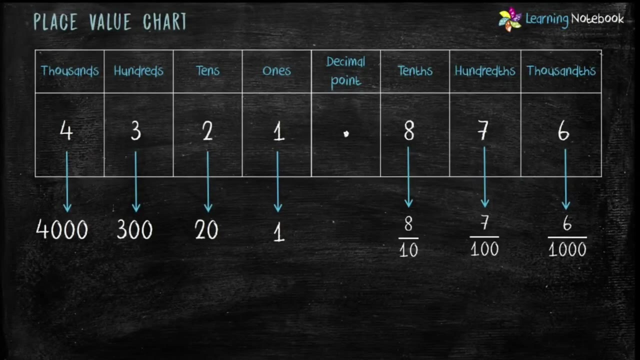 Now let's see the decimal part. Place value of 8 is 8 by 10,. place value of 7 is 7 by 100 and 6 is 6 by 1000.. Now we have got the place. 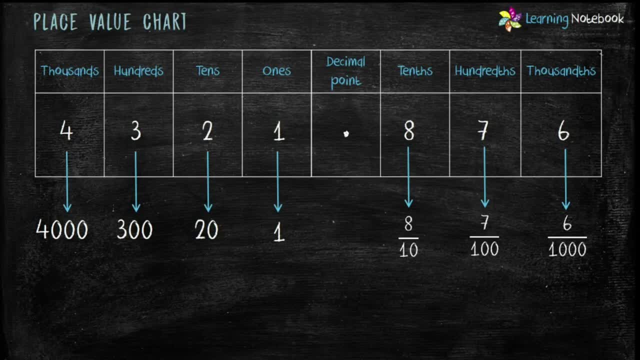 Place value of all the digits of this decimal number. Therefore, its expanded form would be 4000 plus 300 plus 20 plus 1 plus 8 by 10 plus 7 by 100 plus 6 by 1000.. Students note that the decimal number 4321.876. 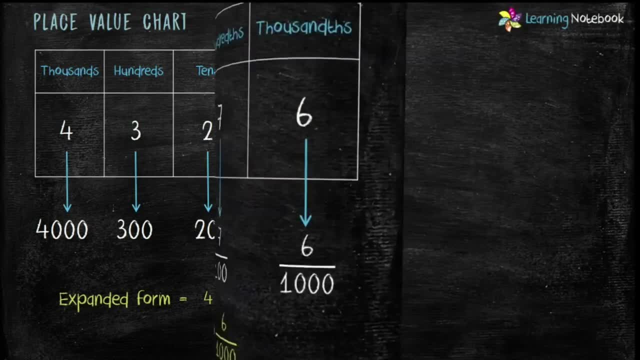 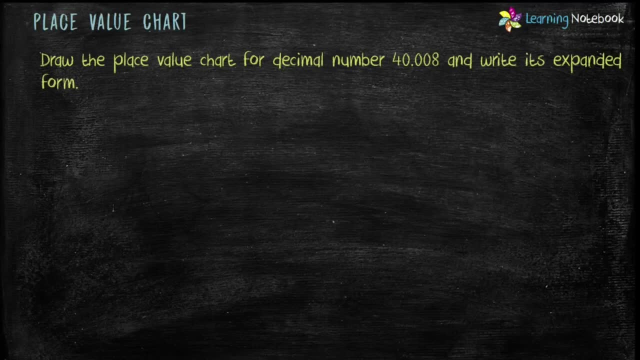 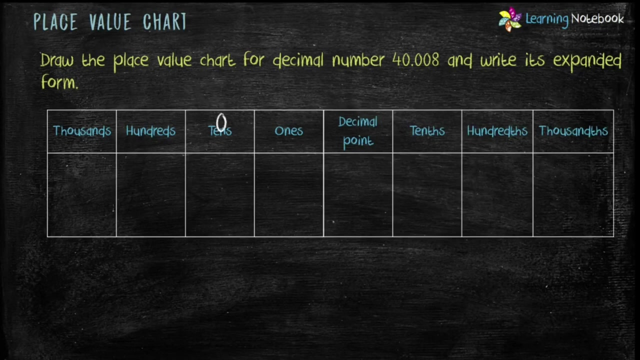 is called the short form. Let's do one more question. Draw the place value chart for decimal number 40.008 and write its expanded form. First let's make the place value chart of whole number part, which is 40. So let's put 0 at 1's place and 4 at 10's place. 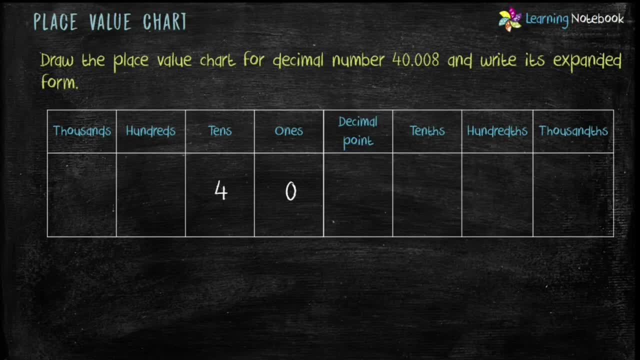 Now let's start with the decimal part. Put a decimal point, Then write 0 at 10's place, another 0 at 100's place and 8 at 1000's place. So, students, this is the place value chart for the given decimal number. 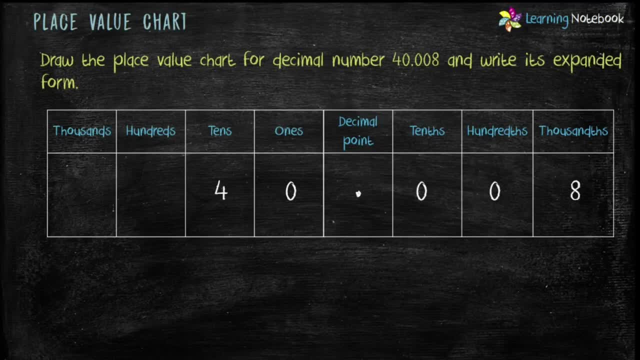 Now to write expanded form. let's find the place value of all these things. Place value of 0 is 0.. Place value of 4 is 40.. Now let's see the decimal part. Place value of 0 is 0.. 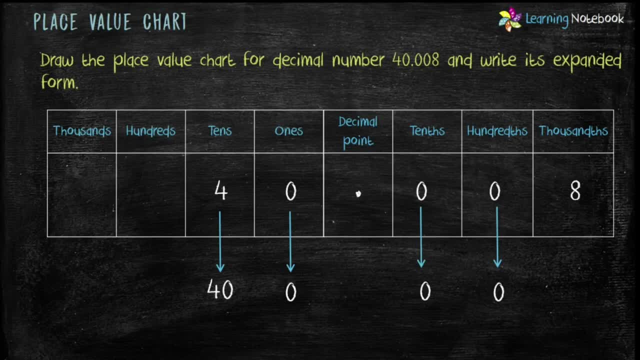 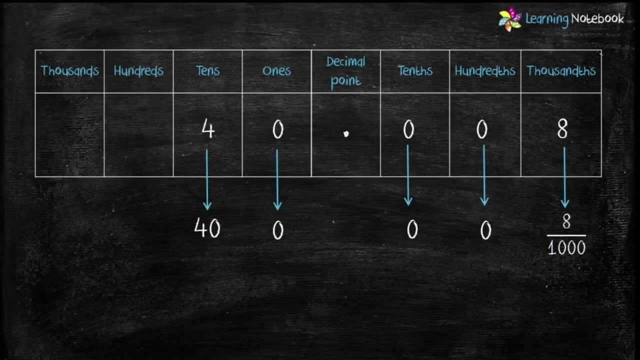 Place value of 0 is again 0.. And place value of 8 is 8 by 1000.. So, students, now we have got the place value of all the digits, So let's write it expanded form, Which is 40 plus 8 by 1000.